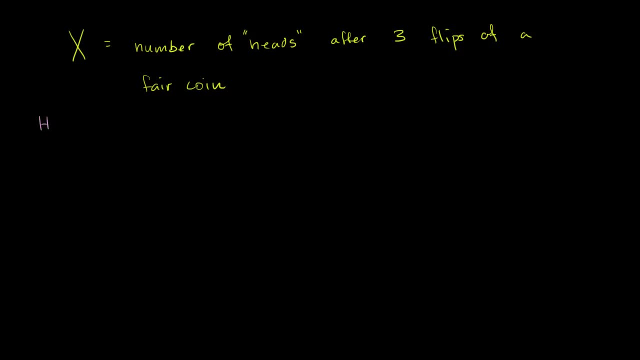 So you could get all heads, heads, heads heads. You could get heads heads tails. You could get heads tails, heads, You could get heads tails tails. You could have tails heads head. You could have tails head tails. 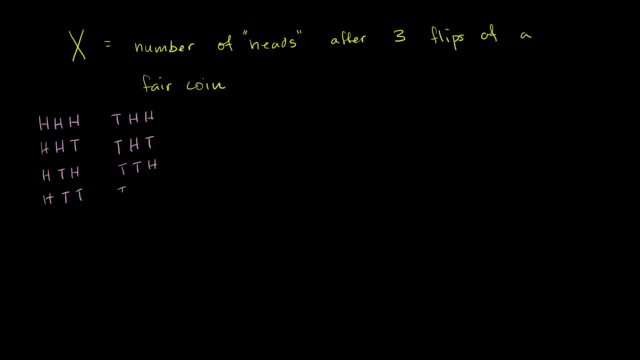 You could have tails, tails, tails, tails, tails, heads, and then you could have all tails. So there's eight equally when you do the actual experiment. there's eight equally likely outcomes here. but which of them? how would these relate? 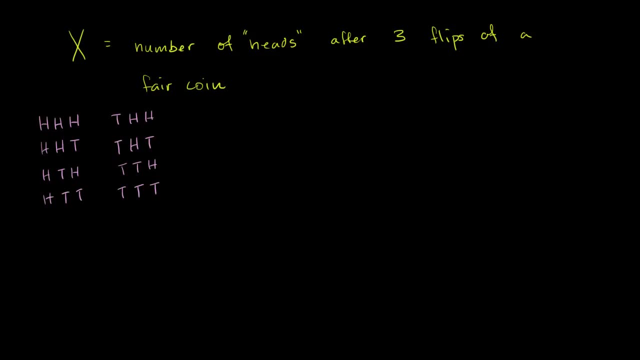 to the value of this random variable. So let's think about what's the probability. there is a situation where you have zero heads, so we could say: what's the probability that our random variable x is equal to zero? Well, that's this situation right over here. 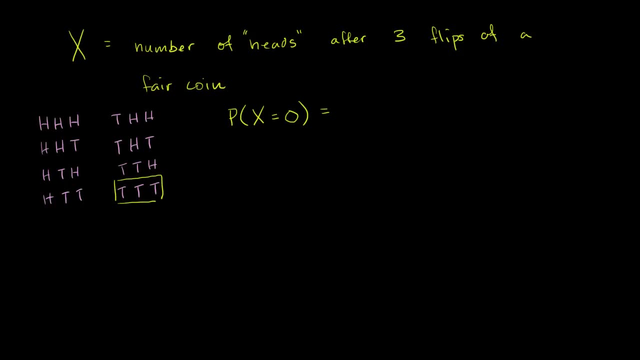 where you have zero heads. it is one out of the eight equally likely outcomes. so that is going to be. that's going to be one over eight. What's the probability? what's the probability that our random variable capital X is equal to one? 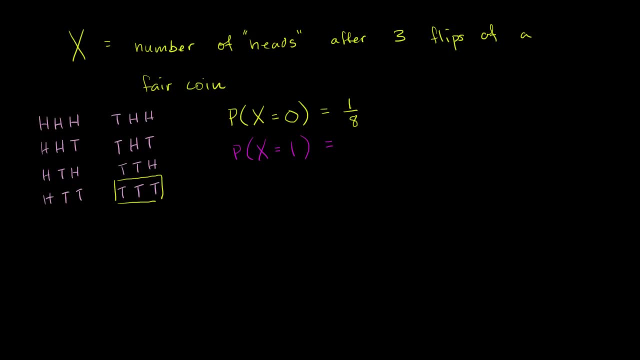 Well, let's see which of these outcomes gets us exactly one head. We have this one right over here, we have that one right over there, we have this one right over there, and I think that's all of them. So three out of the eight equally likely outcomes. 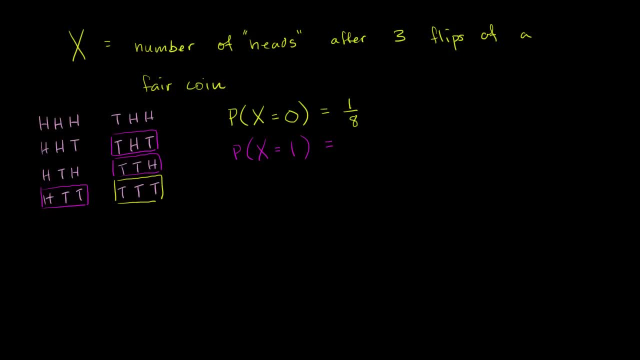 are provide us, get us to one head, which is the same thing as saying that our random variable equals one. So this has a three-eighths probability. Now, what's the probability? and I think you're getting maybe getting the hang for it at this point. 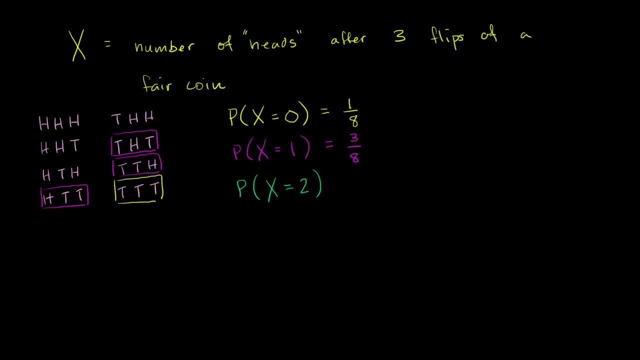 what's the probability that our random variable X is going to be equal to two? Well, for X to be equaling two, that means we got two heads when we flipped the coin three times. So that's: this outcome meets that constraint, this outcome would get our random variable. 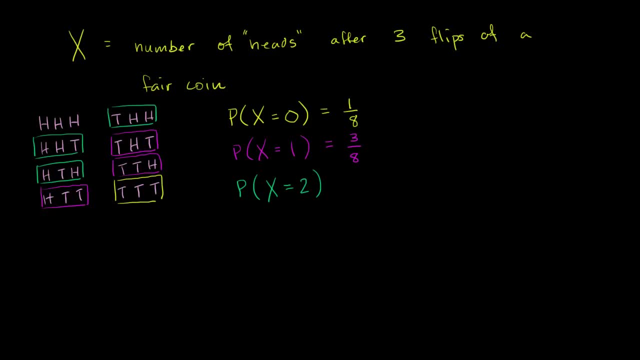 to be equal to two, and this outcome would make our random variable equal to two, and this is three out of the eight equally likely outcomes. so this is a three-eighths probability. And then, finally, we could say: what is the probability? 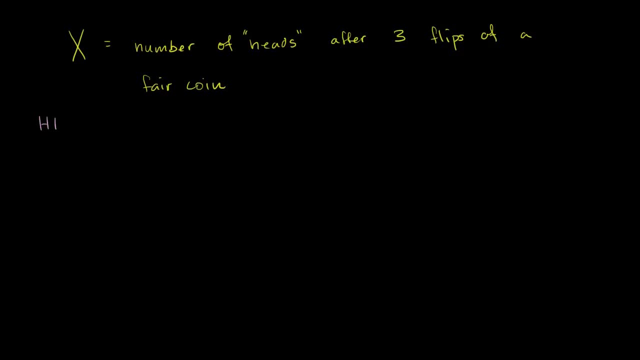 So you could get all heads, Heads, Heads Heads. You could get Heads Heads Tails. You could get Heads Tails Heads, You could get Heads Tails Tails. You could have Tails Heads Head. 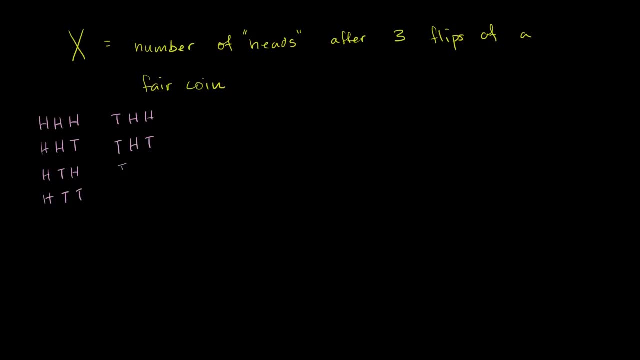 You could have Tails, Head, Tails, have tails, tails, heads, and then you could have all tails. So there's eight equally when you do the actual experiment. there's eight equally likely outcomes here. But which of them? how would these? 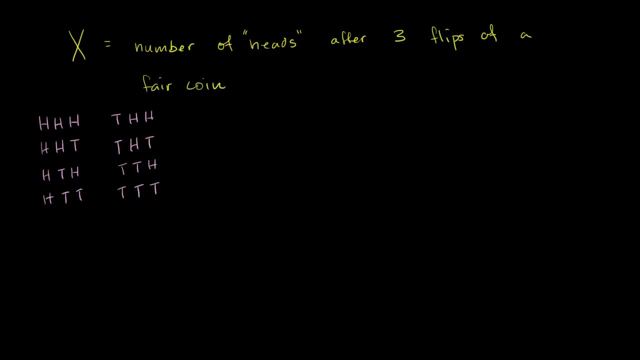 relate to the value of this random variable. So let's think about what's the probability. There is a situation where you have zero heads, So we could say: what's the probability that our random variable x is equal to 0? Well, that's this situation right over here. 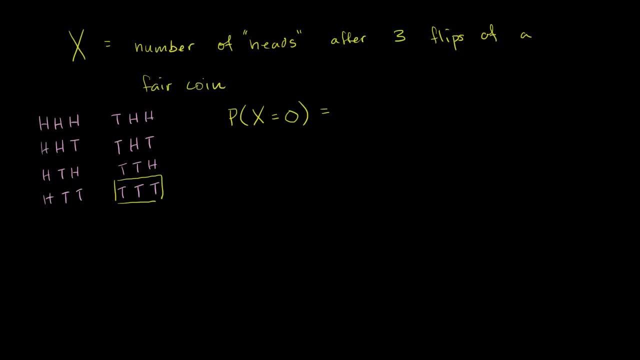 where you have zero heads. It is one out of the eight equally likely outcomes, So that's going to be 1 over 8.. What's the probability that our random variable capital X is equal to 1?? Well, let's see. 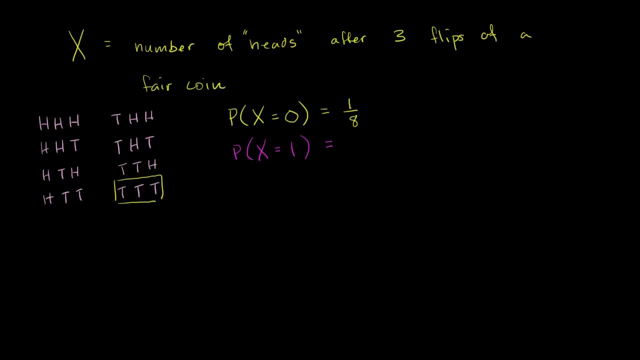 Which of these outcomes gets us exactly one head? We have this one right over here, We have that one right over there, We have this one right over there, And I think that's all of them. So three out of the eight equally likely outcomes. 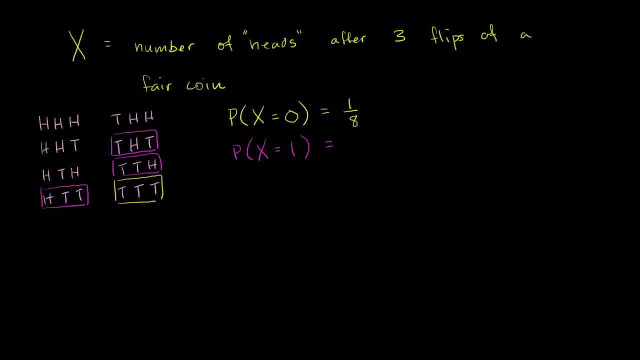 get us to one head, which is the same thing as saying that our random variable equals 1.. So this has a 3 eighths probability. Now, what's the probability? I think you're maybe getting the hang for it at this point. 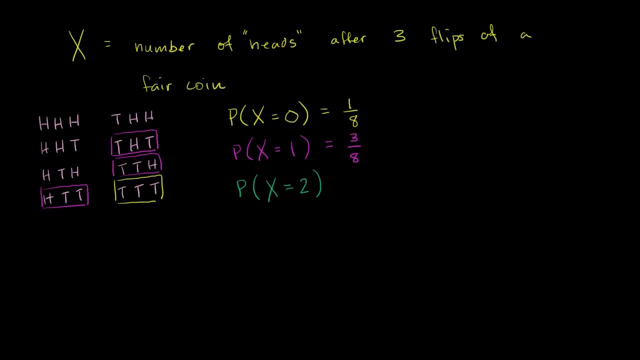 What's the probability that our random variable, x, is going to be equal to 2?? Well, Well, for x to be equaling 2, that means we got two heads when we flipped the coin three times. So this outcome meets that constraint. 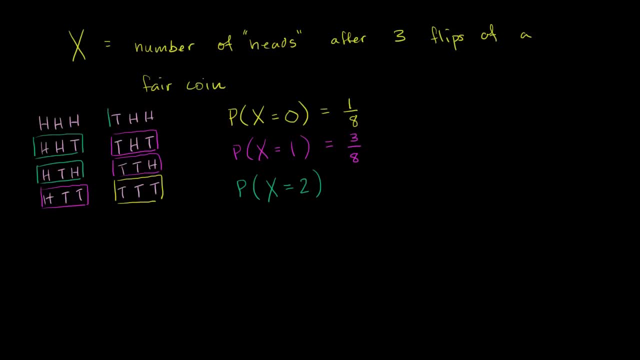 This outcome would get our random variable to be equal to 2.. And this outcome would make our random variable equal to 2.. And this is three out of the eight equally likely outcomes. So this is a 3 eighths probability. And then, finally, we could say what. 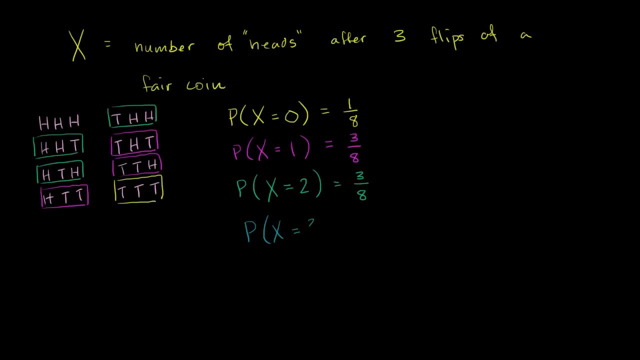 is the probability that our random variable x is equal to 3?? Well, how does our random variable x equal 3?? Well, we would have to get three heads when we flip the coin. So there's only one out of the eight equally likely outcomes. 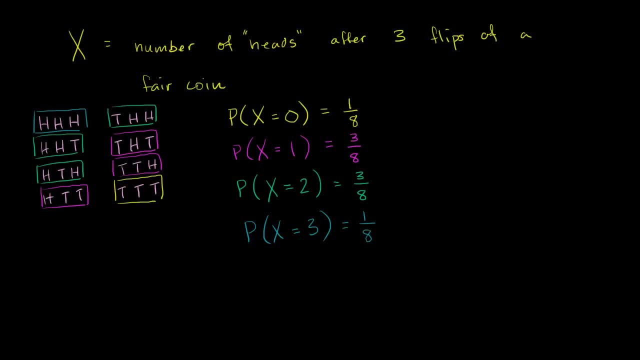 that meets that constraint. So it's a 1 eighth probability. So now we just have to think about how we'd plot this to really see how it's distributed. So let me draw So over here on the vertical axis. this will be the probability and it's going to be between 0. 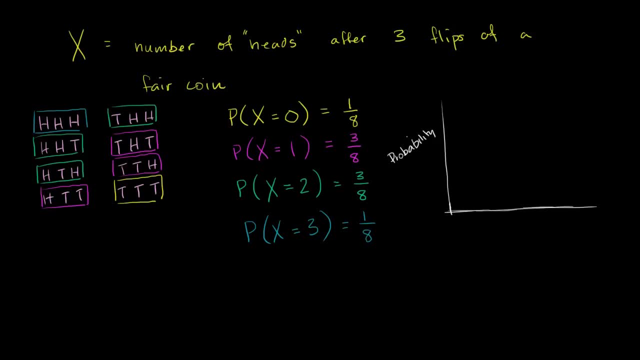 and 1.. You can have a probability larger than 1.. So just like this. So let's see if this is 1 right over here and let's see everything here looks like it's an eighth, So let's put everything in terms of eighths. 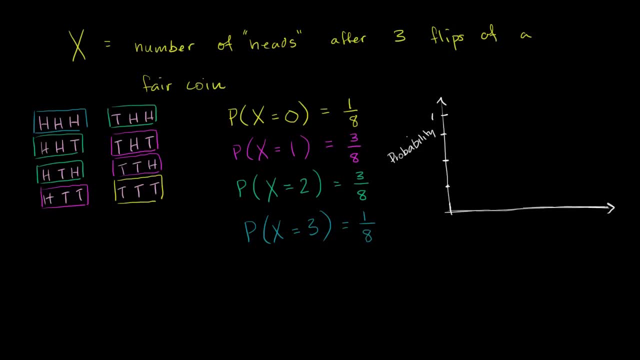 So that's 1 half, This is 1 fourth, That's 1 fourth. That's not quite 1 fourth. This is 1 fourth right over here, And then we can do it in terms of eighths. So that's a pretty good rough approximation. 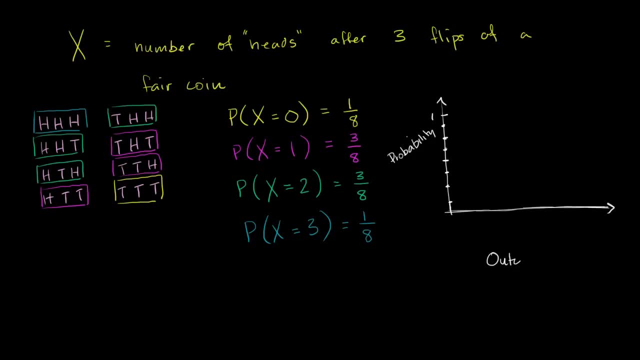 And then over here we could have the outcomes, And so outcomes, I'll say outcomes for let's write this: so value, So value for x. So x could be 0, 1.. Actually, let me do those same colors. 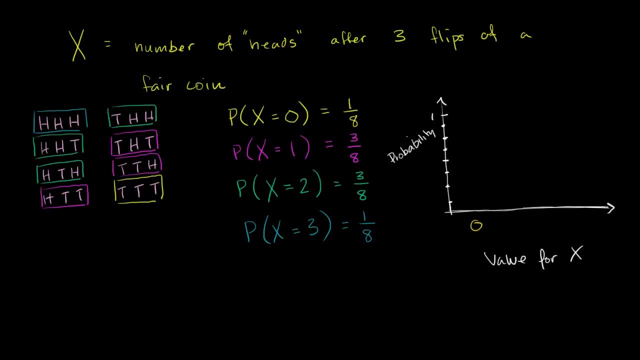 x could be 0.. x could be 1.. x could be 2.. x could be equal to 2. And x could be equal to 3.. x could be equal to 3.. These are the possible values for x. 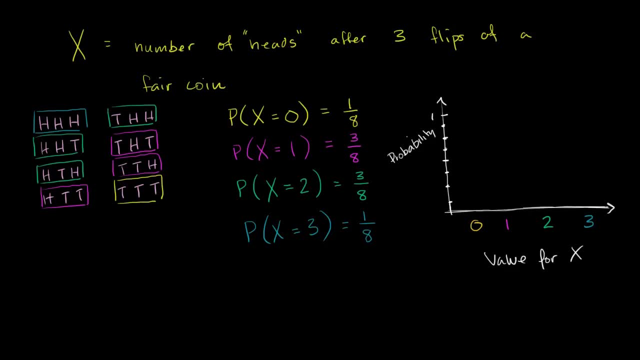 And now we're just going to plot the probability. The probability that x has a value of 0 is 1 eighth. So I'll make a little bar right over here. that goes up to 1 eighth. So actually let me draw it like this: 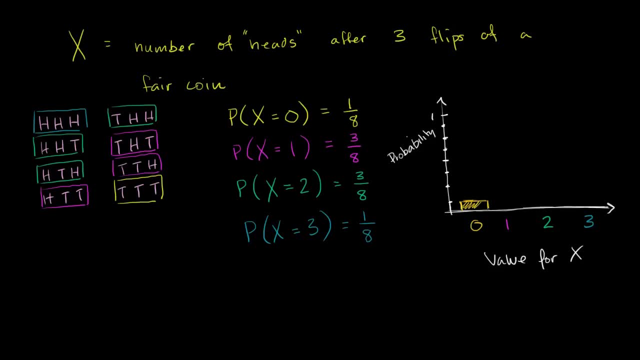 So So it goes up to. so this is 1 eighth. right over here, The probability that x equals 1 is 3 eighths, So that's 2 eighths. 3 eighths Gets us right over. let me do that in that purple color. 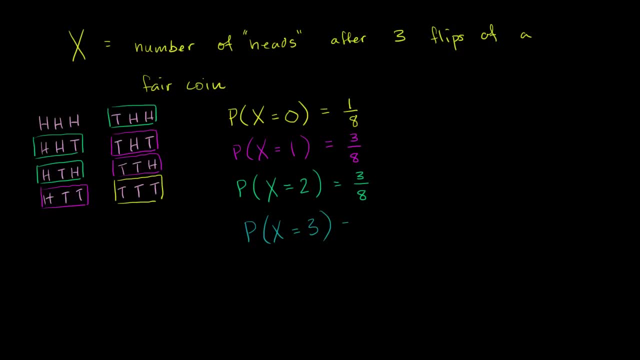 that our random variable X is equal to three. Well, how does our random variable X equal three? Well, we would have to get three heads when we flip the coin. So there's only one out of the eight equally likely outcomes that meets that constraint. so it's a one-eighth probability. 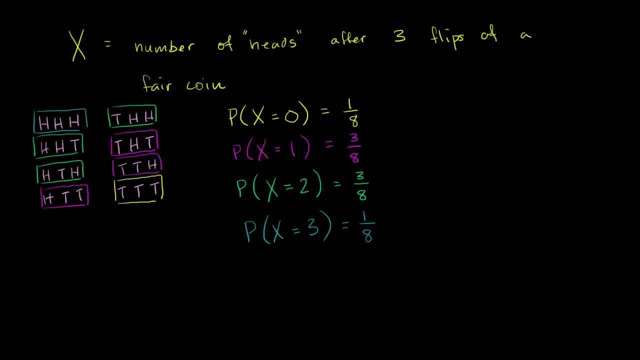 So now we just have to think about how we plot this to really see how it's distributed. So let me draw so over here, on the vertical axis, I'll. this will be the probability probability probability and it's going to be between: 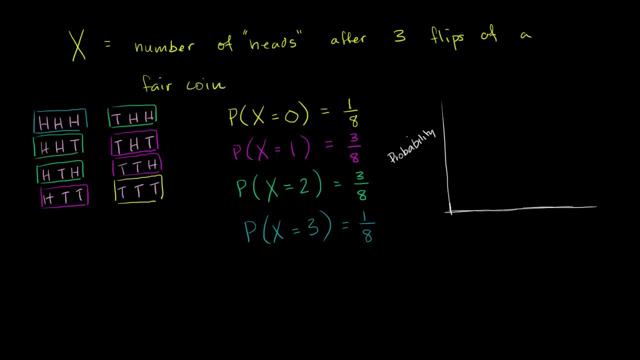 zero and one. you can't have a probability larger than one, So just like this. so let's see if this is, if this is one right over here, and let's see everything here looks like it's an eighth, so let's put everything in terms of eighths. 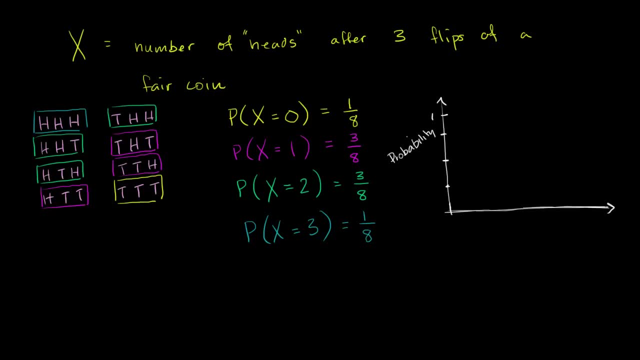 So that's half, this is a fourth, that's a fourth I can. that's not quite a fourth, this is a fourth right over here, and then we can do it in terms of eighths. So that's a pretty good rough approximation. 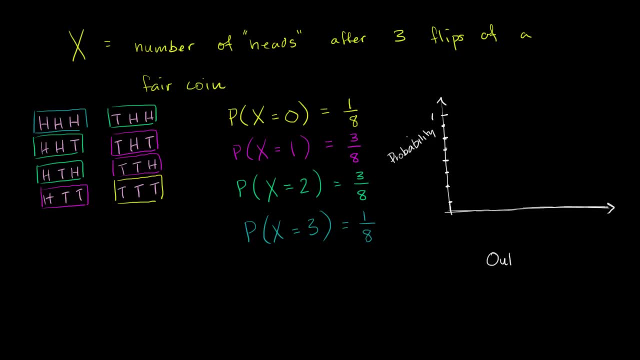 And then over here we could have the outcomes, Outcomes, And so outcomes. I'll say outcomes for, or let's write this: so value, so value for x, So x could be zero one. actually, let me do those same colors: x could be zero, x could be. 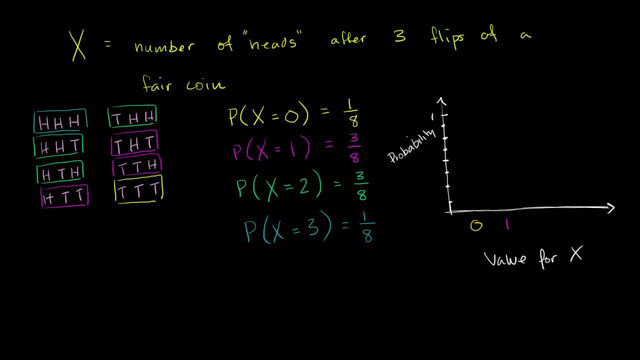 one, x could be two, x could be equal to two and x could be equal to three. x could be equal to three. These are the possible values for x, and now we're just going to plot the probability. The probability that x has a value of zero is one eighth. 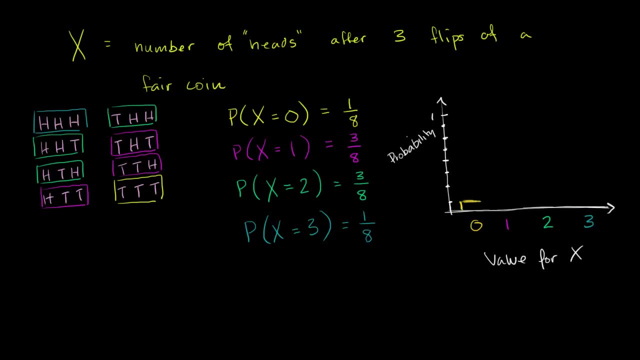 Is one eighth, that's. so I'll make a little bit of a little bar right over here. that goes up to one eighth. So actually let me draw it like this. So it goes up to: so this is one eighth right over here. 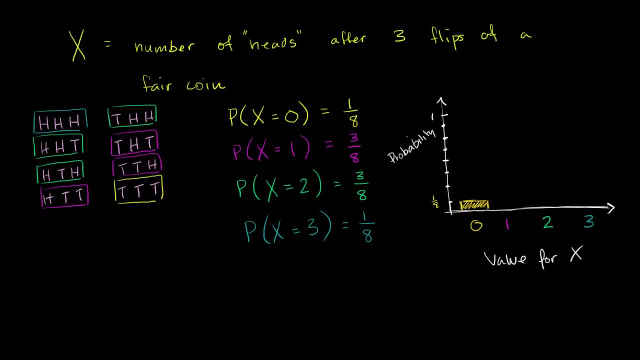 The probability that x equals one is three eighths. So that's two eighths. three eighths gets us right over. let me do that in that purple color. So probability of one that's three eighths. 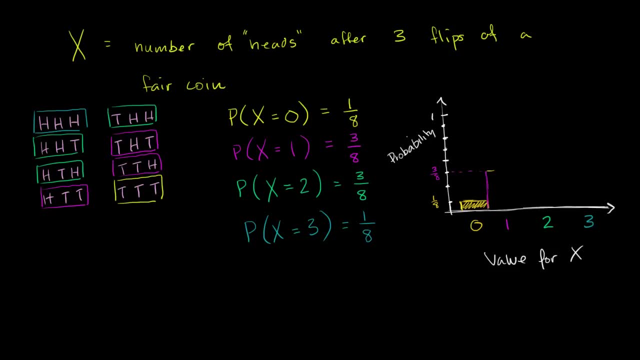 that's right over there. that's three eighths. So let me draw that bar. draw that bar and just like that, The probability that x equals two, the probability that x equals two, is also three eighths. So that's going to be that same level, just like that. 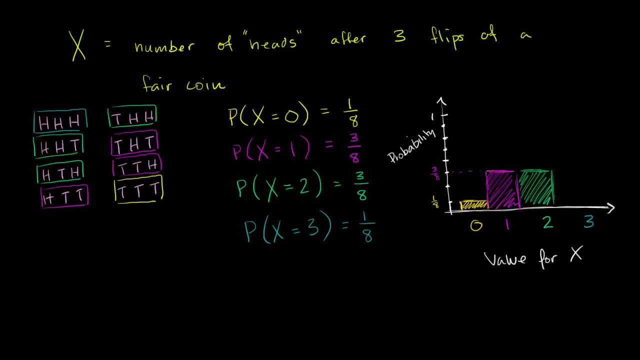 And then the probability that x equals three. well, that's one eighth. One eighth is going to be the same height as this thing right over here, so actually I'm using the wrong color, so it's going to look like this. It's going to look like. it's going to look like this: 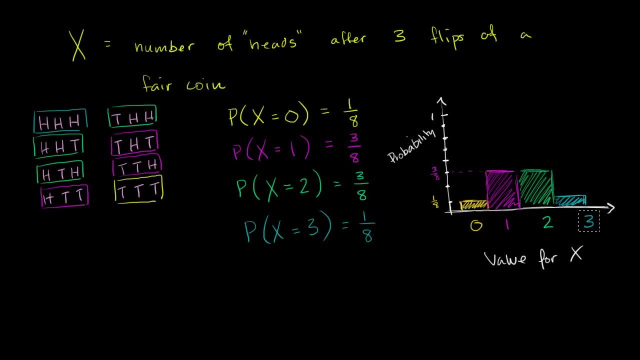 And actually let me just write this a little bit neater. that can move that three. So cut and paste. Let me move that three a little bit closer in, just so it looks a little bit neater and I can move that two in actually as well. 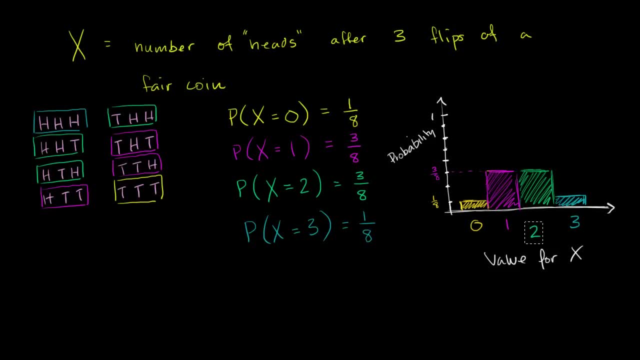 So cut and paste, So I can move that two and there you have it. We have made a probability distribution for the random variable x, And the random variable x can only take on these discrete values. It can't take on the value half or the value pi. 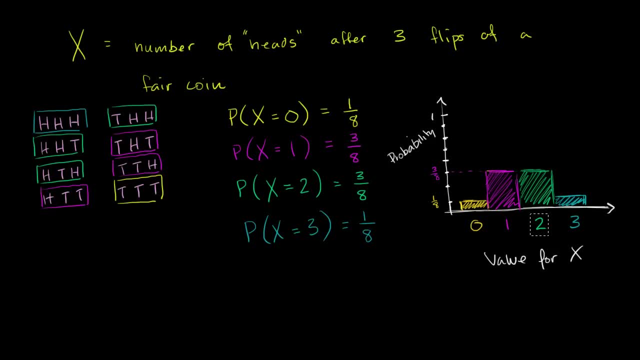 or anything like that. And so this: what we've just done here is we've just constructed a discrete probability distribution. Let me write that down. So this is a. this right over here is a discrete. It only takes the random variable, only takes on discrete values. 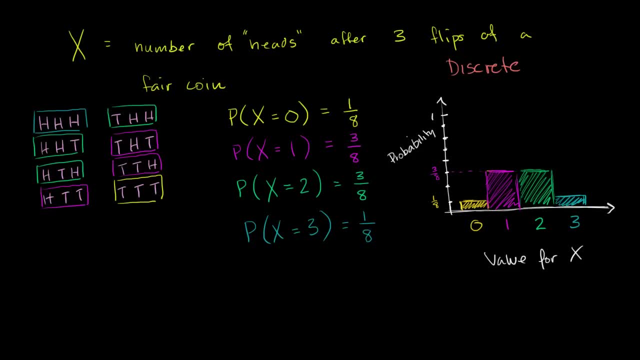 It can't take on any value in between these things. So discrete probability, probability distribution, distribution for our random variable x.